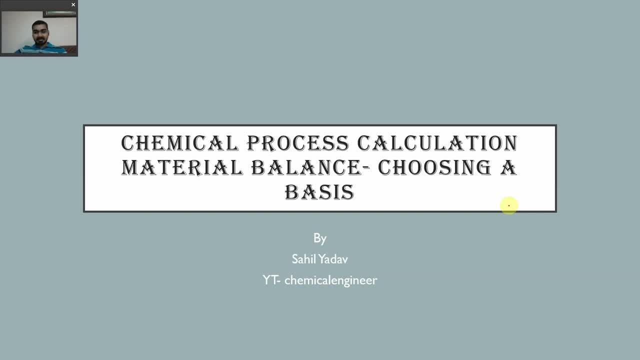 hello everyone, welcome to the channel. chemical engineer. I am Sahil Yadav and I am back after a long time. so continuing to the course, chemical process calculation. so this will be my fourth video in this subject. so in this video we are going to learn about material balance, choosing a basis. so in this video, what we will see, 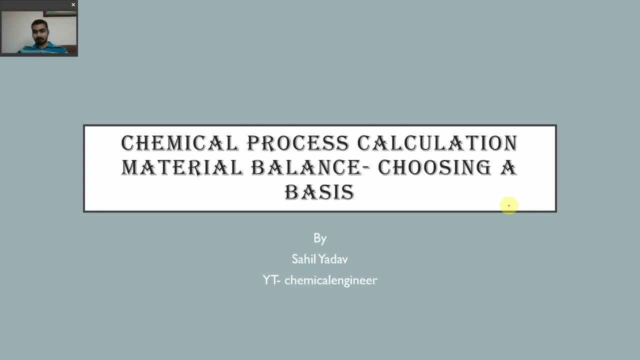 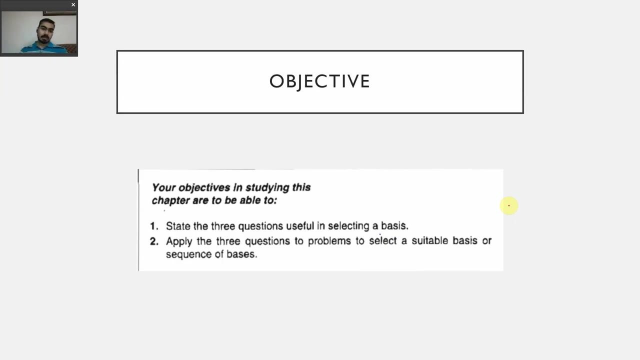 is we will choose a basis. so what is basis and what it is having a relation with problem solving? that all we will see in this video, so please subscribe to the channel. it is my humble request. before starting the video, let us start the video. okay, so choosing a basis. so objective of this video will be to state the three 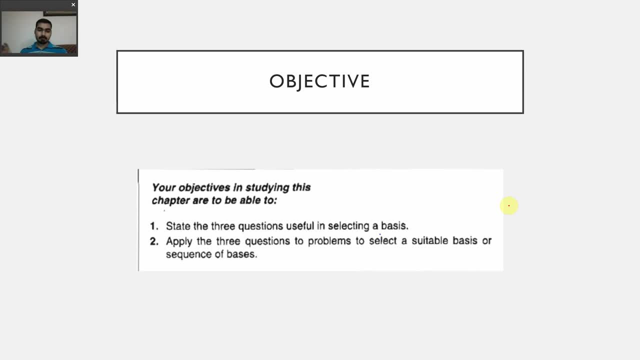 quotients useful in selecting the basis. okay, so there will be three quotients for which you should know how to select a basis for it. okay, and then apply this quotient to select a suitable basis at sequence of basis. okay, so applying this quotient to get the final answer, all right, so those three. 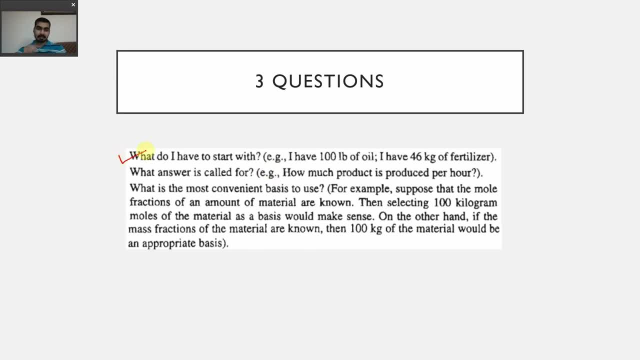 quotients are: what do I have to start with? okay, so if you are given any problem, you should know how to start it with. you may be given much more or wide range of details in your quotient, like. suppose you are given a question like: suppose this is a one quotient. suppose I have hundred pound of oil as well as I. 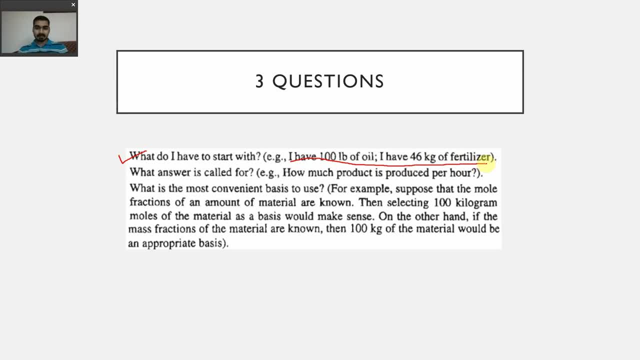 have 46 kilogram of fertilizer or, let us say, 46 kilogram of oil. okay, so, if you are given this, two sentence in one quotient, which should be your appropriate basis, so okay. so basis, so basis is nothing but something which is predefined by us, which is given to us. 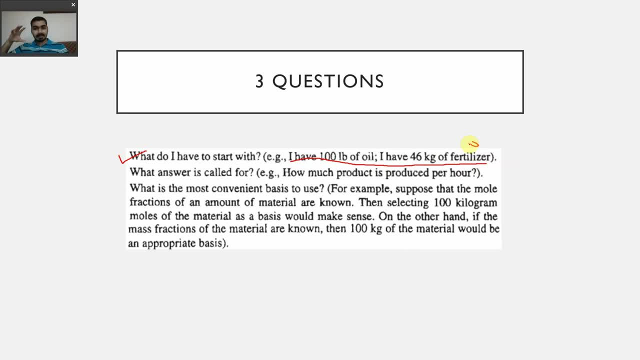 in a quotient. so, taking it as a base, we are going to solve a problem, so that is known as basis. okay, so you should know how to start it. then what answer is called for means you should know what is our aim. to select that basis or what is. 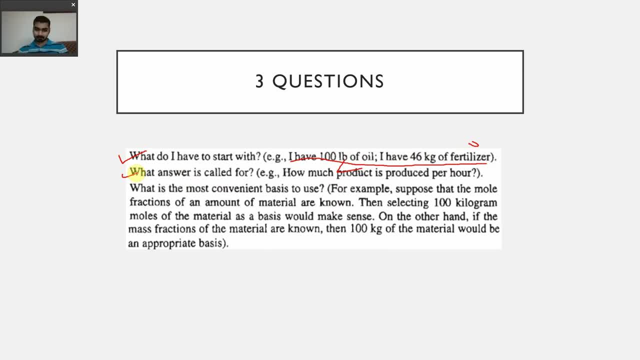 our aim to find out in the quotient, okay, so in the quotient you will be given something like: find out the mass fraction, mole fraction, find out the ratios or anything like that, how much product flow rate. anything will be given to you, so you should know what you. 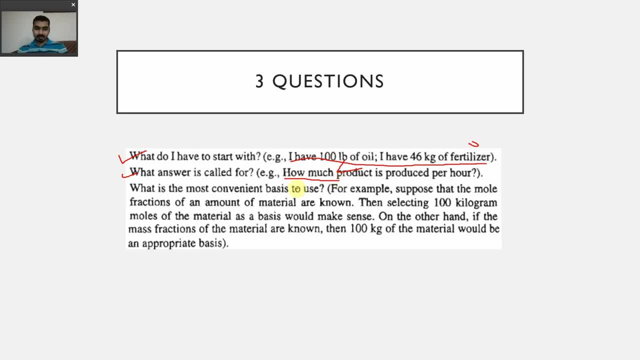 have to find in your answer. okay, and then the third quotient, which is the most important quotient. you should always use it while starting or writing the answer. so what is the most convenient basis to use? as I have discussed in the first question that you will be given more, 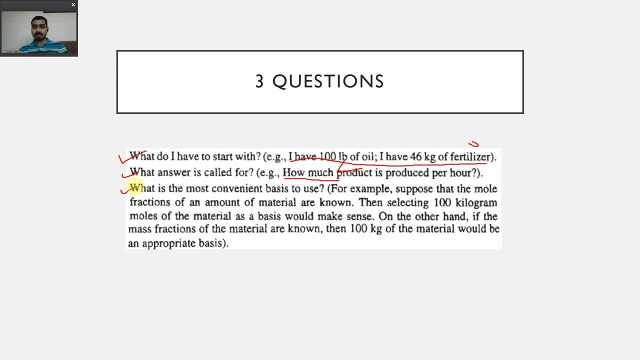 than one data in your quotient. so which data should you use or choose as a basis? on this, on the type of basis or on the base of the basis, we are going to solve the next part of the problem? okay, and that's it. we have to answer these three. 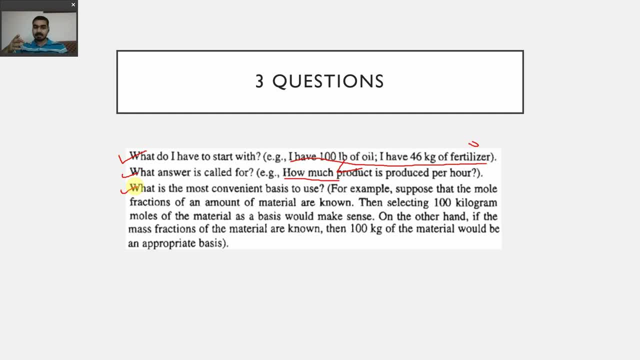 questions or if we know how to apply basis. we will get the answer for these three questions. so before going to the examples, let me tell you, in process calculation, if you are given any quotient, any quotient in process calculation, if you are given first line, you should write is basis. so suppose, if you are, we will see an example. but what you 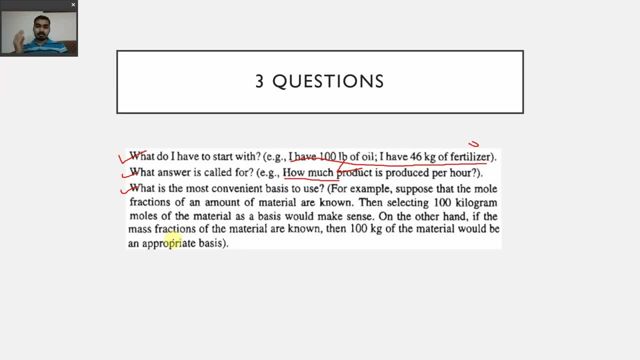 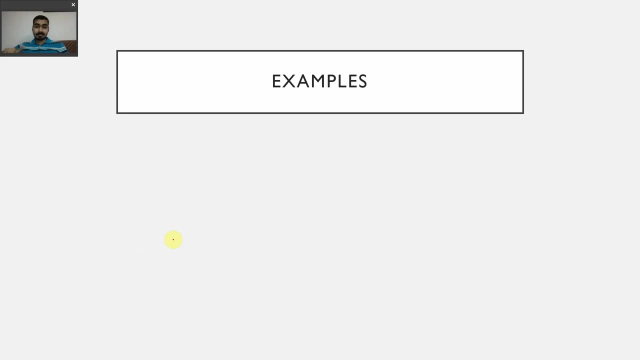 have to write first line of any question should answer of your answer should start with basis dash, so dash will be. i will explain you by looking at the examples. all right, and yeah, this is a process calculation. yes, the name suggests calculation. always keep your pen paper in your hand and solve it side by side. pause the video and solve it, all right. 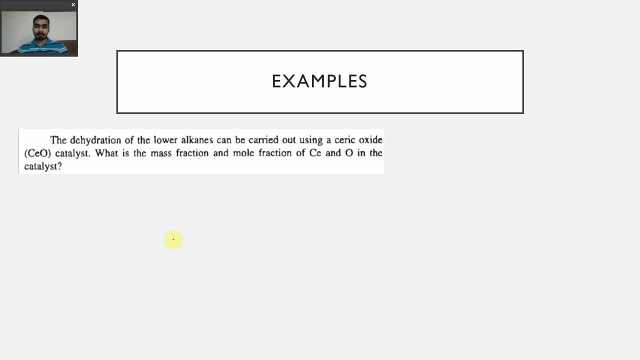 so the choosing a basis is the main aim. okay, remember. so the first question is: the dehydration of lower alkyds can be carried out using a oxide ceo catalysis. what is the mass fraction on the mole, fraction of ceo in the catalysis? all right, so you know anything about cerium oxide or cirric oxide? no, 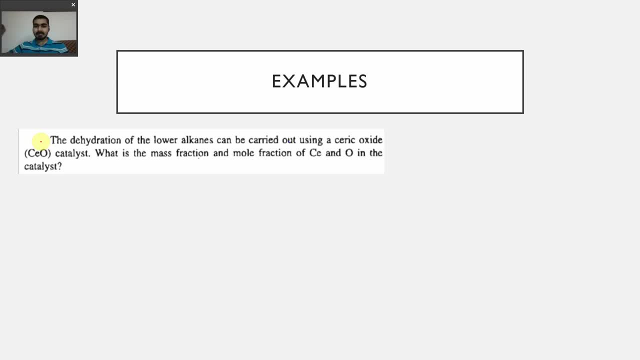 all right. so you have nothing in your brain about this. so how to start with? all right. so, as we know that ceo is formed from cerium, that is, c and oxygen o. so what is the final formula? ceo. so what we can write is, being the chemical engineer, you should be doing it- that cerium plus. 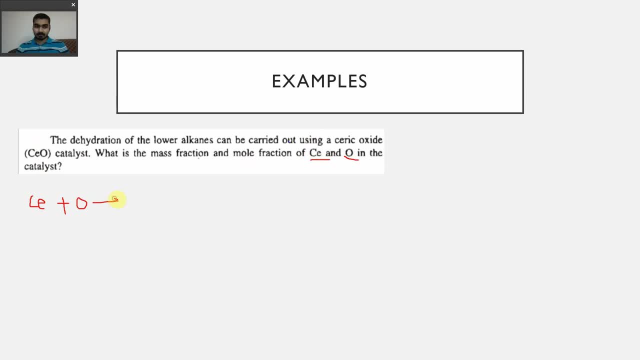 oxygen. we are not taking it as o2, we are just not knowing anything. we are just dumb, so like that. we can write it in a simple way: as ceo is formed by reacting c and o, all right, let us suppose this is one gram. uh, one kilogram, let us suppose, because kilogram is the good unit to use, and this is also one kilogram. 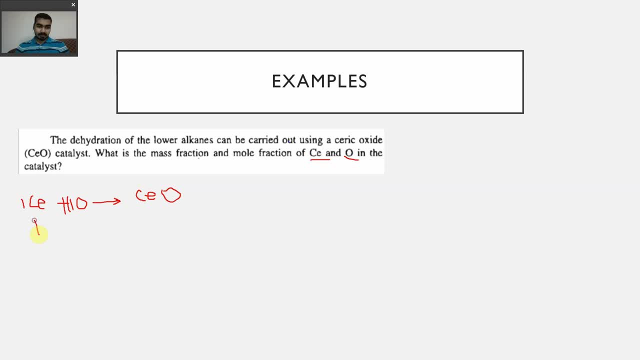 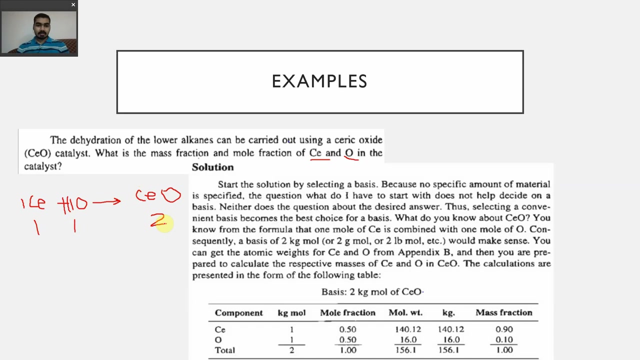 so the total product will be okay. so this is one kg, one kg. so total product: one one will be two kg. all right, done, all right. so this is the first intuition that should come in your mind after looking to the question like this. now let us see the solution. 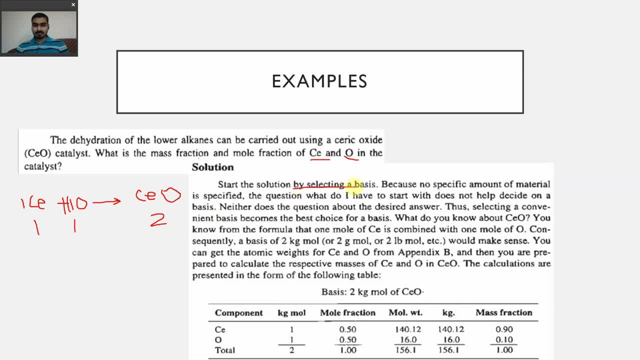 so first line should be selecting a basis, but here, as equation is not given, we have to first write equation. so, because no specific amount of material, we specified the question: what should i start with? is the quotient? all right, so we have written this equation. that is ce plus o gives ceo. so this is the 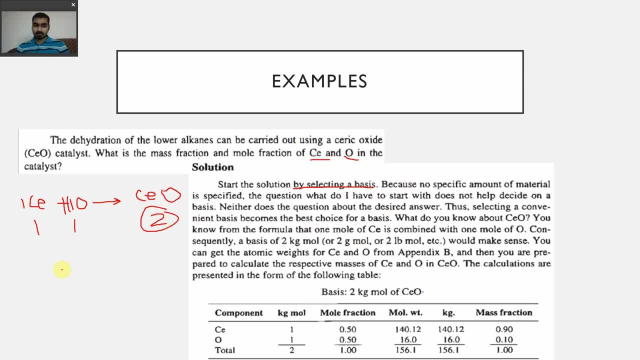 two kilogram. so we can write the equation. can choose a basis of 2 kg. okay, on the basis of mass we can choose this 2 kg. or else one mole of cerium plus one mole of oxygen will give you two moles of cerium oxide- clear. so 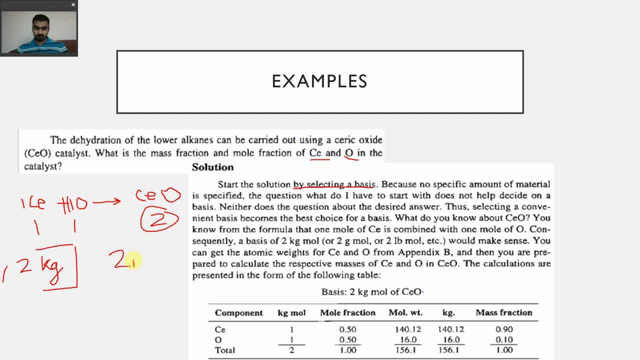 we can use two mole of cerium oxide as a basis, all right, so now we have two bases. now what you should do? you have to choose one basis. so read the question again: what is the mass fraction and mole fraction of cerium and oxide in catalyst? 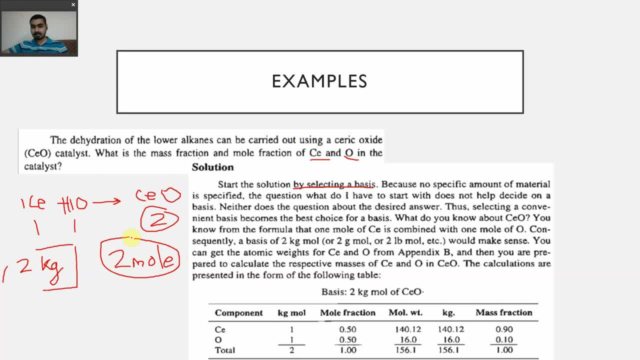 so which thing is easier to find? think about it then. all right. so let me tell you: the easiest thing is mass fraction, because you will be knowing the mass of cerium and mass of oxygen. both you will be knowing. so mass fraction can be calculated easily, can choose a basis as two mole, because that is what unknown quantity which we are assuming in. 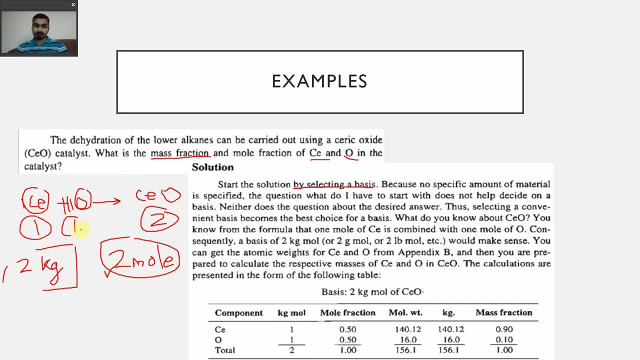 this equation by taking as one mole. one mole gives two mole. as such, there is no direct relation. also, that one kg of cerium plus one kg of oxygen will give you two kg of cerium oxide. so the best thing to choose is two moles, all right, this is how you have to eliminate and do this step in just one. 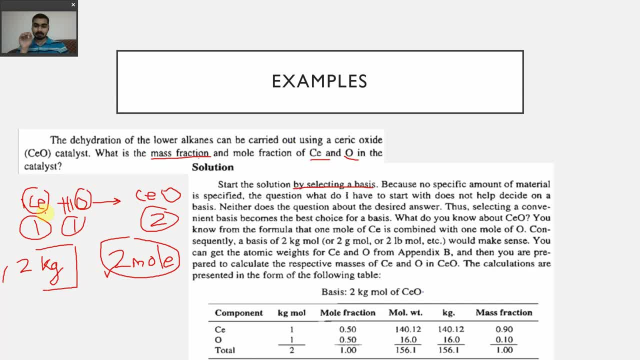 minute or less than 30 second in your exams. all right, done so we will choose two more of this ceo as our basis. so then you have to make a table, or if you are not making a table, you should clearly know how to write. so one mole, one mole gives two mole of cerium oxide. this is our first. 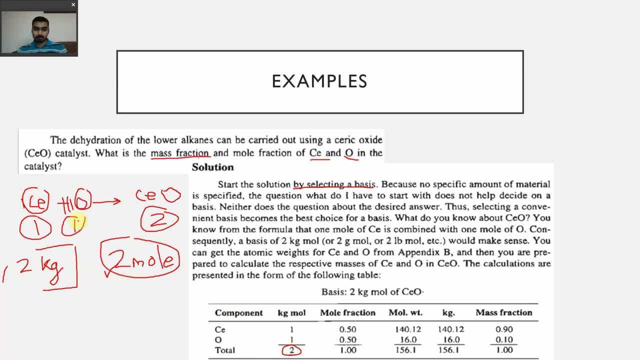 step mole fraction. so this is one by two and oxygen is also one by two. so one by two and one by two. point five, point five: total will be one molecular weight- you should be knowing of both of them, kilogram. so as one molar present, kilogram and molecular weight will be remaining same done. 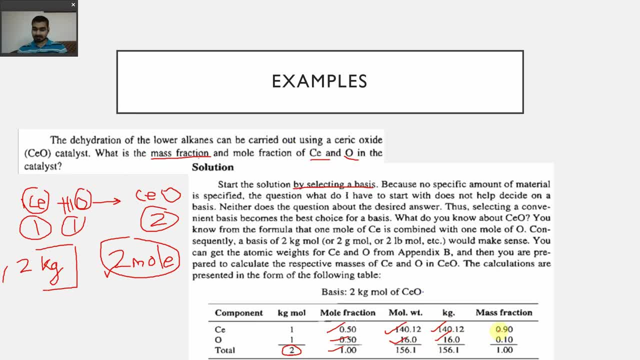 mass fraction. how are you calculating now mass fraction? simple: 140 by 156.1 will give you the mass fraction as 0.8, and 16 by 156.1 will give you the mass fraction as 0.1. simple how to select the basis is clear. i should assume that you should be. 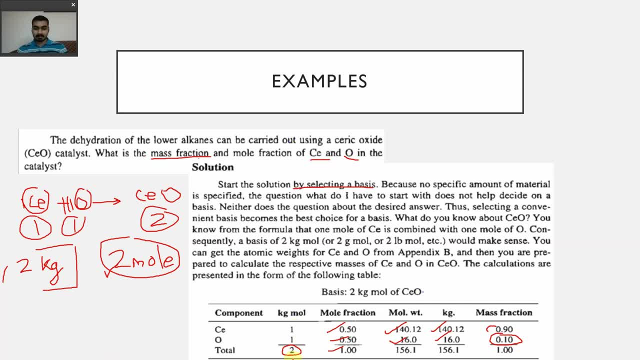 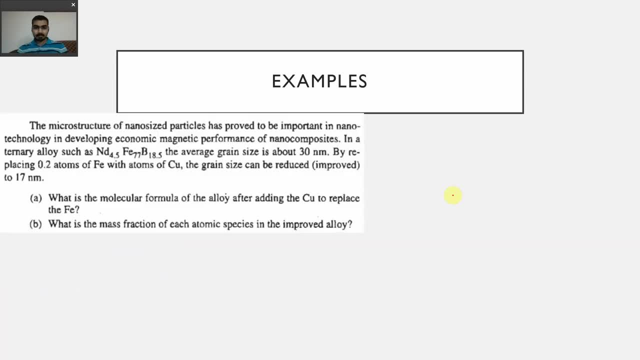 clear by now that how to select that basis. all right, this is the second and the last example for this video. so the microstructure of nano size particle has proven to be important in nanotechnology in developing economic magnetic performance in nano composite in a ternary alloy. 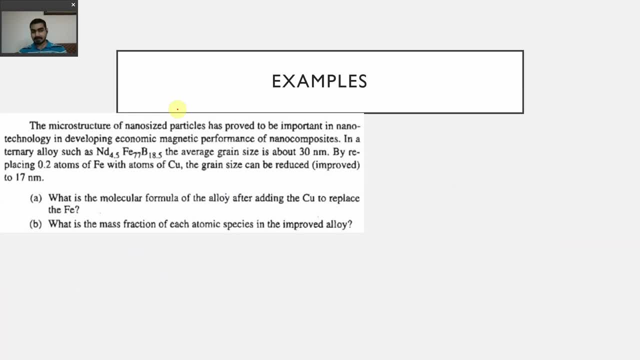 such as nd 4.5- ferrous 77- boron 18.5, cd4, and in a ternary alloy, such as nd 4.5- ferrous 77- boron 18.5, the average grain size is about 30 nanometer. by replacing 0.2 atom of iron with atom of cu. 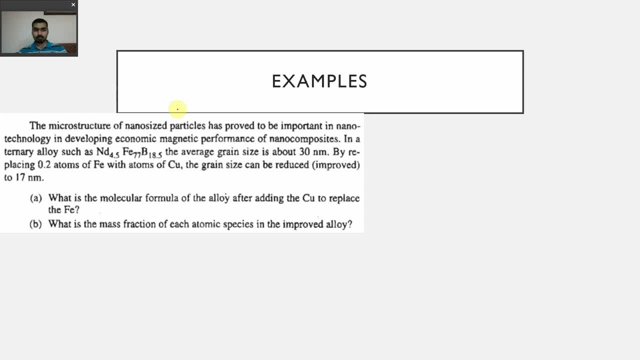 the grain size will be can be reduced to 17 nanometer. all right, don't read the a and b part. so what you are given is, first thing is this formula: size, size, and this is the final size and the condition you have. you are given is: 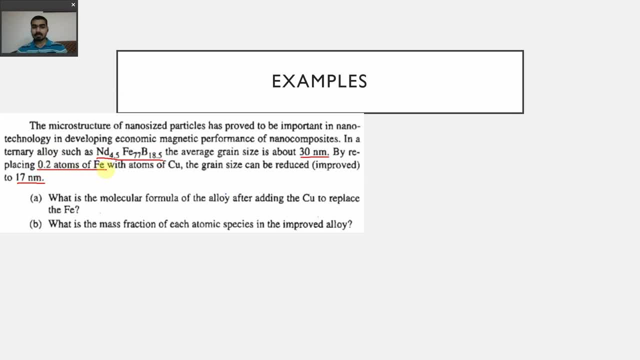 you have to replace 0.2 atoms of iron with copper. all right, done these. all things are given okay. so what should be your basis? think about it. done, all right. so you should carefully observe this question. you are given atoms what it has mentioned: 0.2 atoms of. 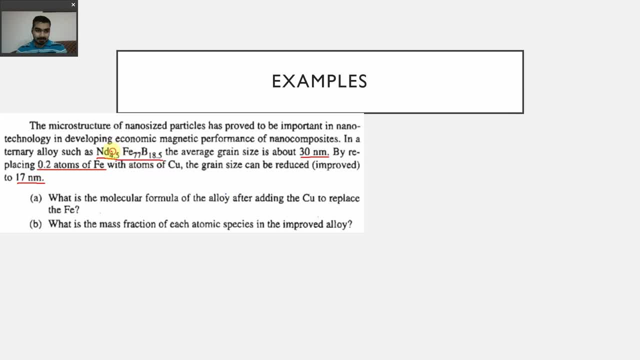 iron means all these values, that is, 4.5, 77 and 18.5 are the atoms. all, right, and carefully observing, you will come to know that 77 plus 18.5 plus 5 are the atoms right, you have to carefully observe. 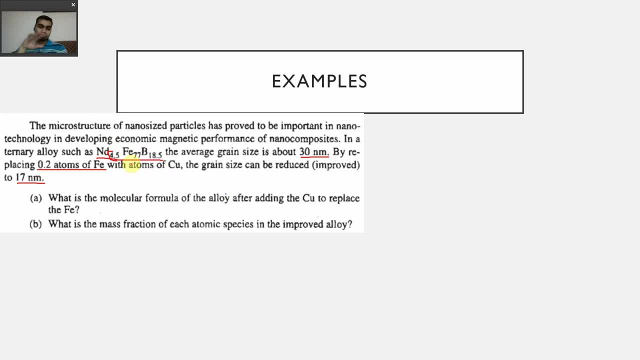 4.5 will become, will become 100. so what we are changing, that is atoms. we are manipulating atoms. so our basis should be in terms of atom only. why? because that, if the basis is in terms of atom, because that is the only thing we are given in the quotient, we are given size. 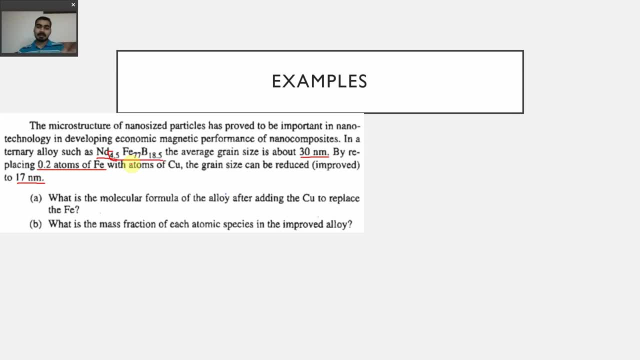 but that is varying where a variable- so we can't choose it as a basis basis- should be a permanent, or we can say the thing with by which we can get other data as well. so that is how you should choose a basis. so here we will choose hundred atoms of an. what is this? 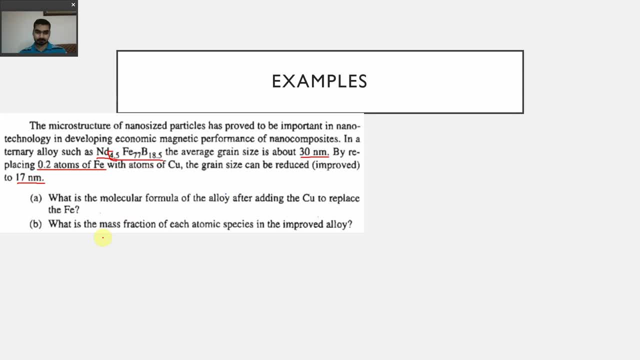 alloy. okay, so that should be your basis. what is the first question? now, basis is selected. now read the quotient: what is the molecular formula of alloy after adding the copper to replace iron? okay, so we are given, to manipulate point, two atoms of iron. so we will subtract point. 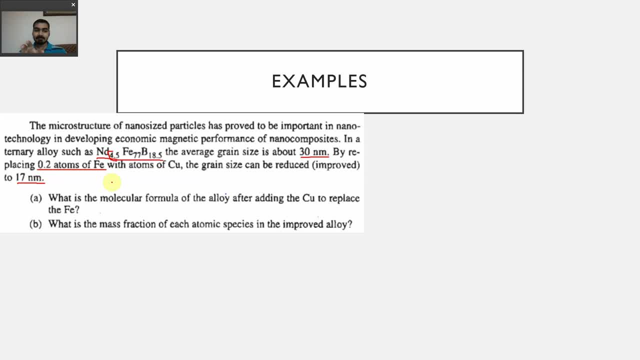 two atoms. so what we will get for iron seventy seven minus point two, that is seventy six point eight, and we are adding copper, so new formula will be nd four point five, iron seventy six point eight, boron eighteen point five into copper. let me see: okay, copper is okay. so copper is zero point two, because 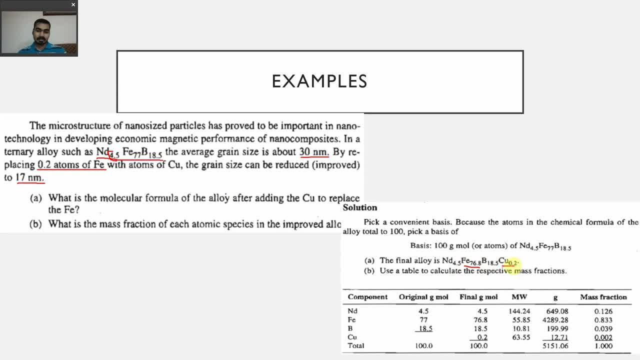 that is what. iron is removed, copper is added. so this will be a final alloy formula: what is the mass fraction of each species or in the will be: what is the mass fraction of each species or in the? That is based on the present value of the unit number, which is this. so, in this case, 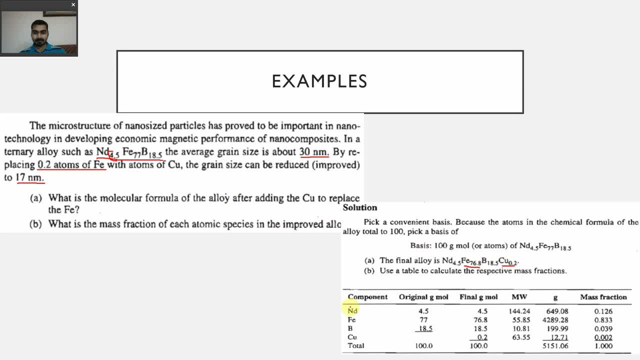 or in the improved element, simple mass fraction. 100 is our original gram mole, 77 and 18.5 is our initial 100. final atoms are 4.5, 76.8, 18.5 and 0.2. total will be 100 as well now. 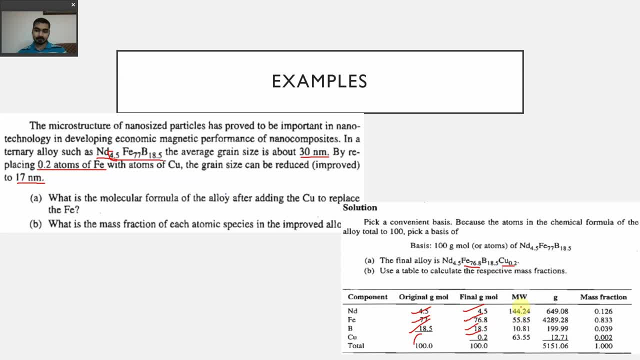 you are given a molecular weight, molecular weight will be given to you, or else you can find it any book. so these are our molecular formula. molecular formula or molecular weight multiplied by gram, you will get equivalent weight, or we can say the gram actually. so multiply molecular weight. multiply by that is 144 into 4.5, you will get 649, and so on. 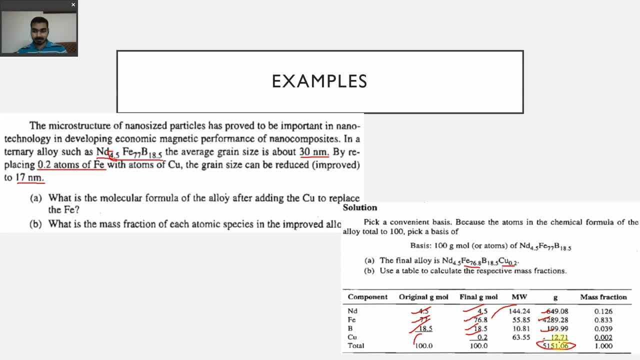 so total value will be provided, or we will get the total value will be provided and then will get directly: five one five, one point zero six. divide each six, forty nine point zero eight, divided by five one, five, one point zero six, you will get the mass fraction of nd fe b. so for b, 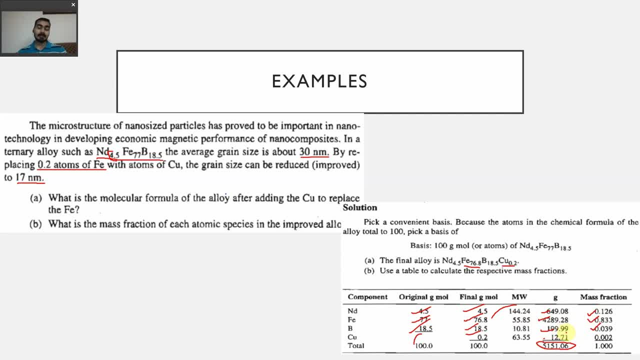 will be nineteen, one, ninety, nine point nine divided by one. uh, five, one, five, one point zero six. so this is how you can calculate the mass fraction. is it simple? in your exam, nothing more than this will be going to be asked, okay, so you have to have clear knowledge. how to 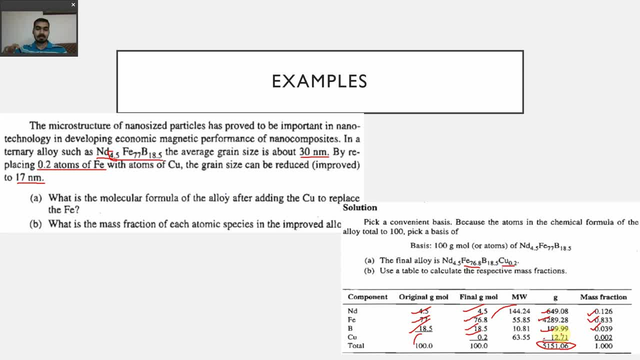 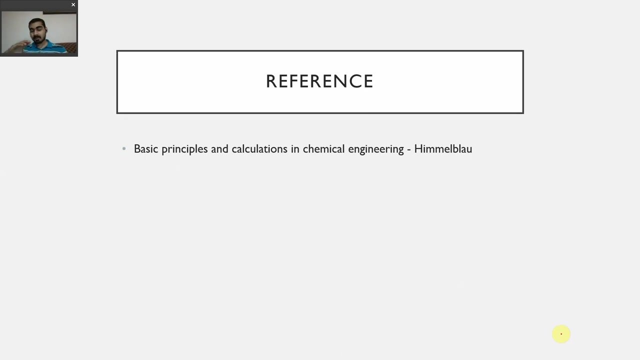 select a basis. if you still have a doubt, you can just comment or you can contact me through telegram, instagram, anywhere. okay, there is concept of changing a basis, so that concept we will learn while solving a numerical questions. okay, in the next videos, for reference or not for a reference, you should.